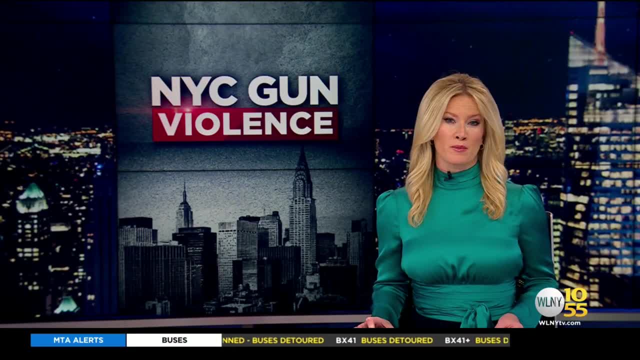 Well, victims and community leaders announced a new partnership to try to help stop gun violence in the city. It's a campaign called Boycott Black Murder. CBS2's Christina Phan has the details: Boycott Black Murder. Boycott Black Murder. 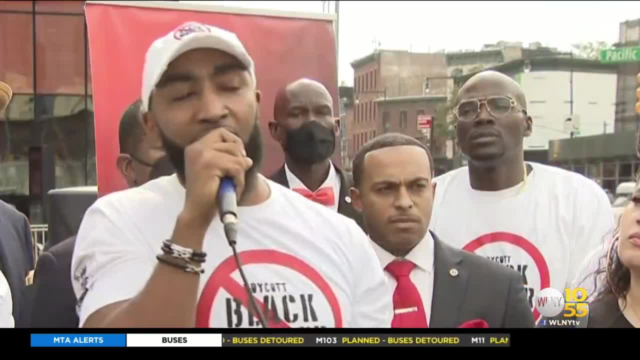 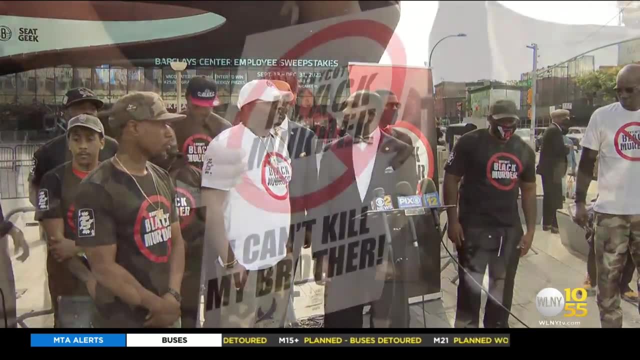 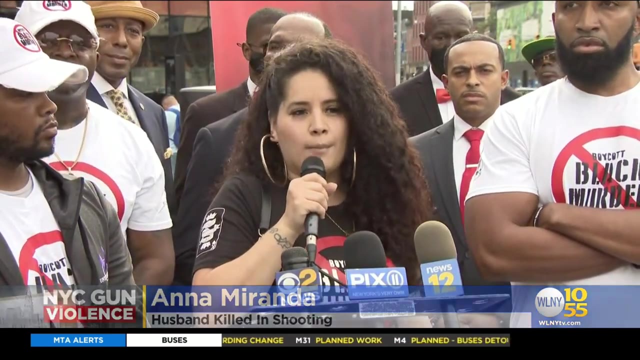 Victims of gun violence, the formerly incarcerated and those just tired of the endless bloodshed, gathered in front of the Barclays Center Saturday, coming together to launch a campaign called Boycott Black Murder. The community is tired. We are emotionally drained. We've experienced so much trauma over the years. 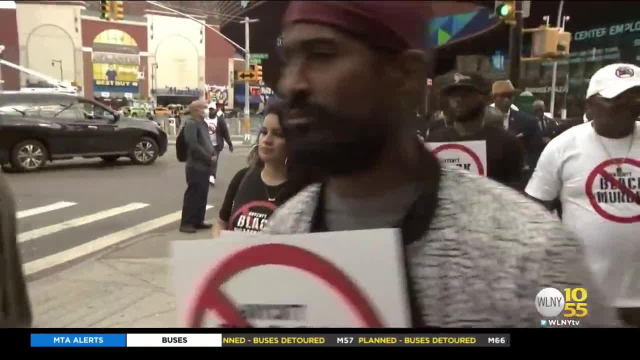 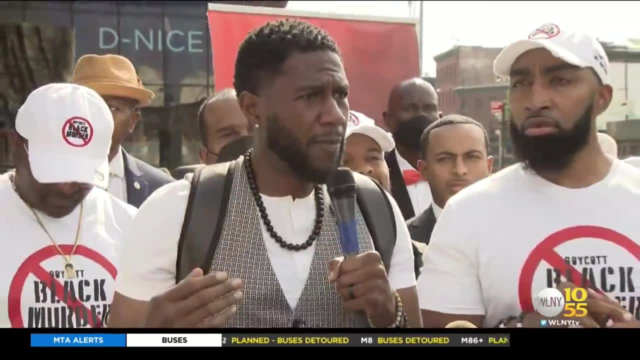 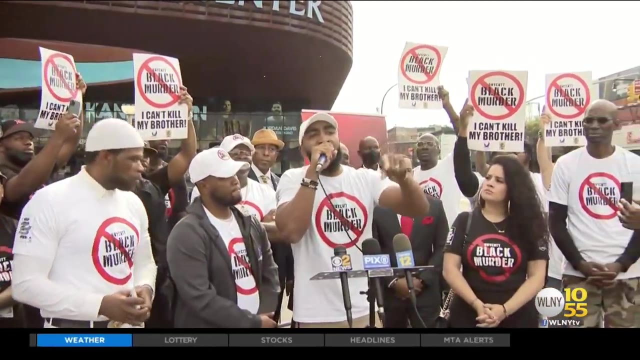 Alarmed by the rise in children getting killed by guns, a coalition of community advocacy groups gathered to announce a new partnership between violence interrupters, elected officials and families to saturate the most impacted communities and demand support from local businesses as well as social media platforms. 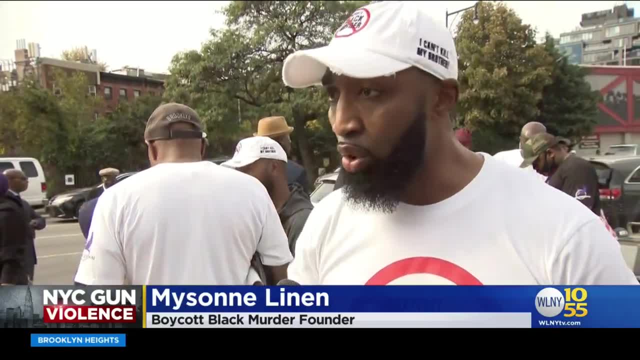 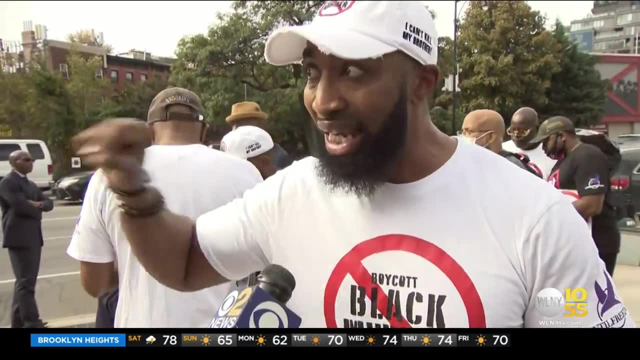 I want to utilize those relationships to advocate for this work. to promote this work The same way you would promote a Wu-Tang Clan tour, we're going to promote Boycott Black Murders tour. We're going on a tour to each individual project. 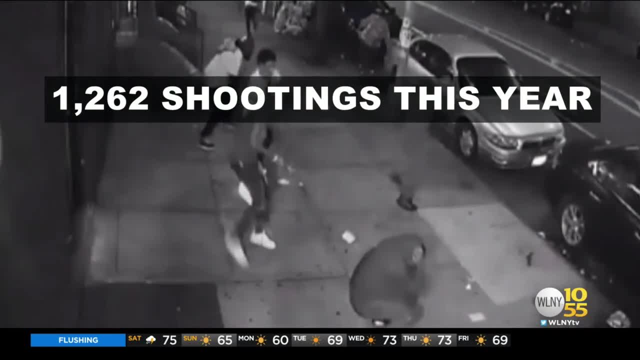 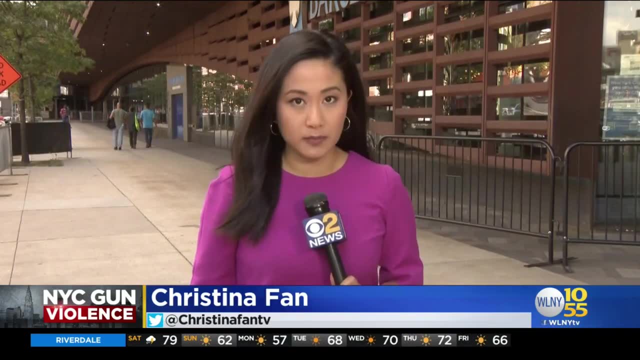 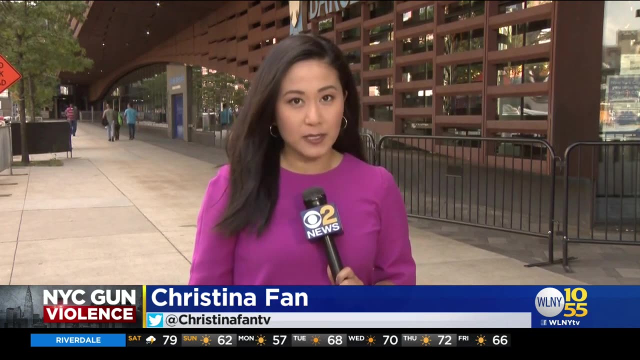 According to the NYPD, there's been at least 1,262 shootings this year, with 1,517 victims. Public advocate Jumaane Williams says the key to decreasing these statistics is by giving less funding to police and by giving more resources to community advocacy groups that have been proven to work. 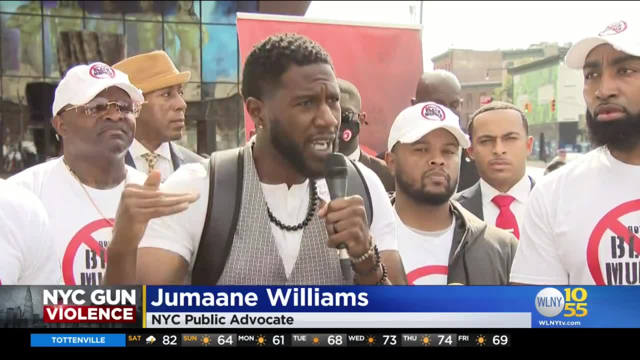 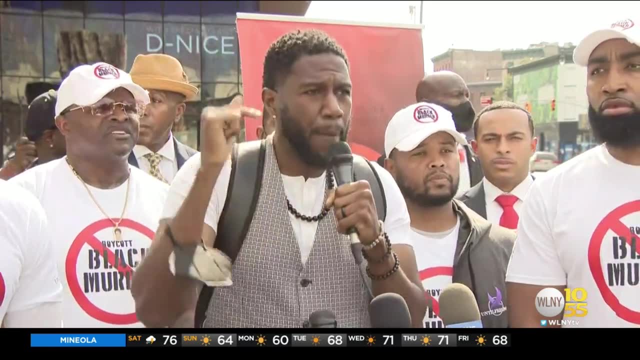 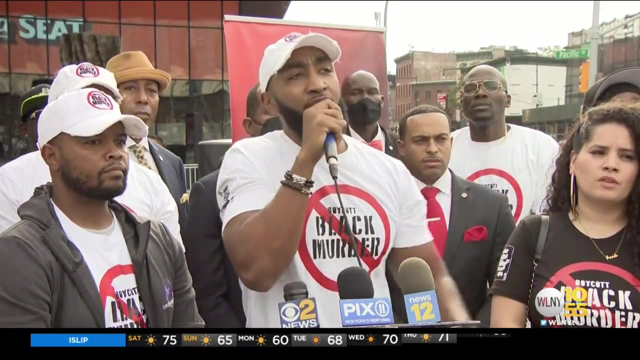 We cannot equate public safety simply with policing. All we're asking is for the rest of the things that create public safety in communities to be funded and put in the infrastructure. We're telling everybody that you have to give us the same platform. you've got to give us the same vision, the same publications. 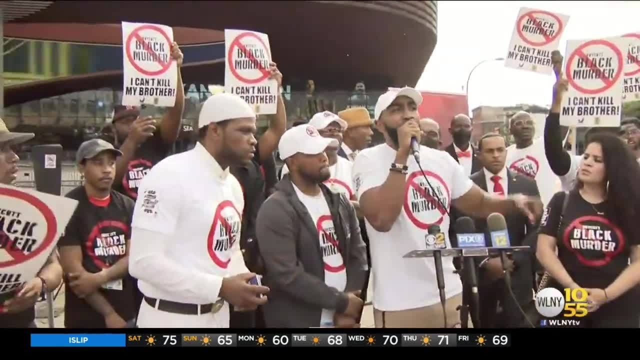 Those who served time for gun violence say they are now leading the charge to solve it At the Barclays Center. Christina Phan, CBS 2 News.